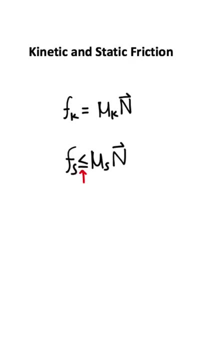 this is your static friction coefficient. Now I want you to pay specific attention to this. less than or equal to sign, And the reason that that's there is because this is not necessarily what your static friction is going to equal. This right here is just: 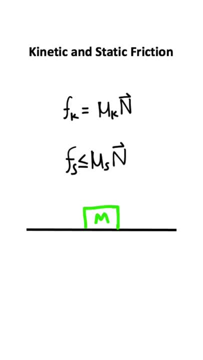 the maximum threshold for static friction. So, for example, if we had a block with some mass and its weight force is going to be mass times gravitational acceleration, and we had a normal force acting up, what we could do is try applying a force to this block. 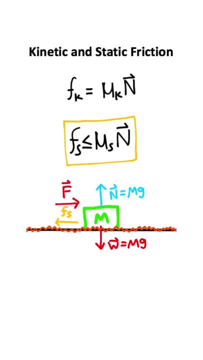 Now, if we had a strong friction on our surface, then static friction is going to oppose this block here equally and make it so this block doesn't move. Even if we applied a greater force, the block still wouldn't move if it didn't break this maximum threshold here. 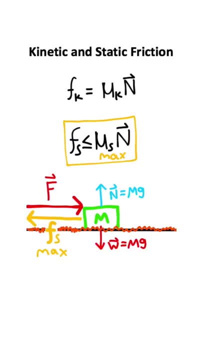 Now let's say that we did actually break past the maximum threshold here and here by applying an even greater force. Well, now what's going to happen is you're going to convert to kinetic friction, which means this block is now in motion. So that's a general introduction to kinetic friction. Introduction to static and kinetic friction. 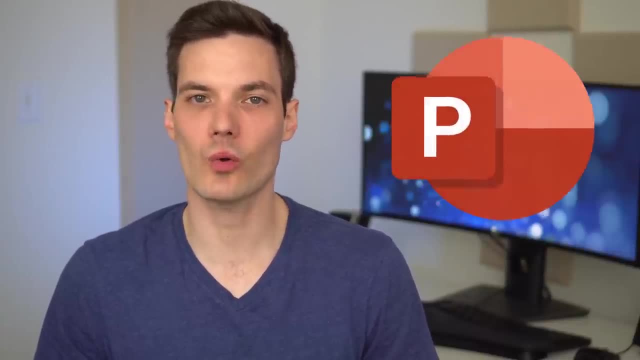 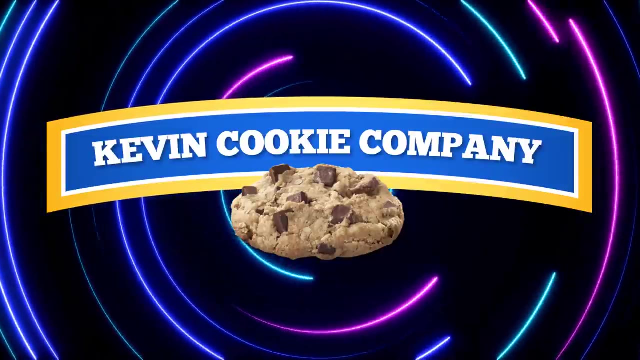 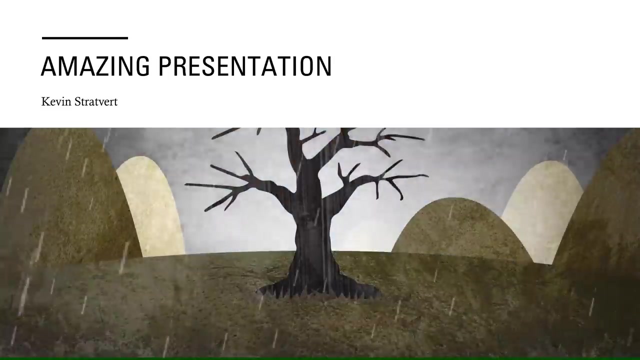 Hi everyone. Kevin, here Today I want to show you a quick trick that's sure to impress any audience. You can insert video backgrounds in Microsoft PowerPoint. The great thing is, you don't have to install any add-ins. As long as you have PowerPoint, you can take advantage of this. 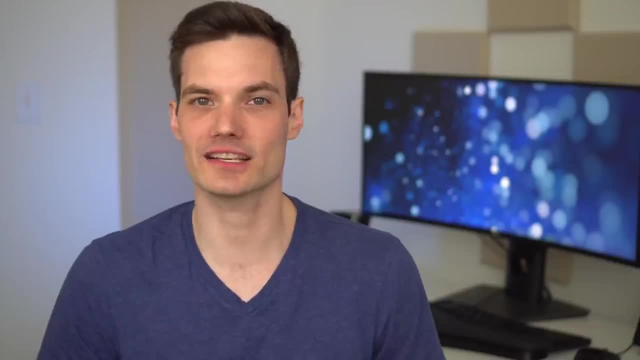 There is one caveat before we jump in. To be able to use this, you need a Microsoft 365 subscription. but if you have that, you are good to go. All right, let's jump on the PC and let's check this out. I'm in Microsoft PowerPoint and I have a blank slide and I'm ready to start inserting. 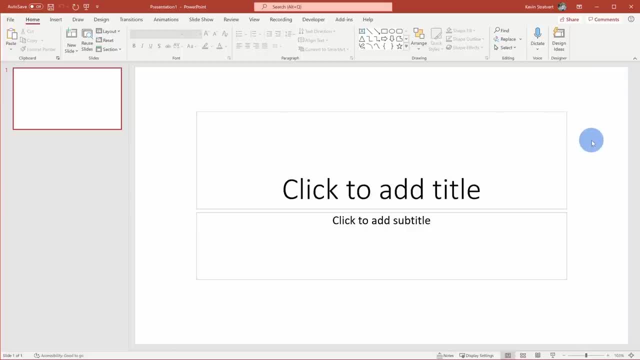 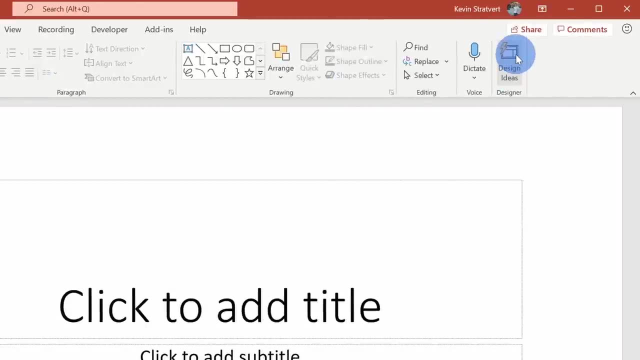 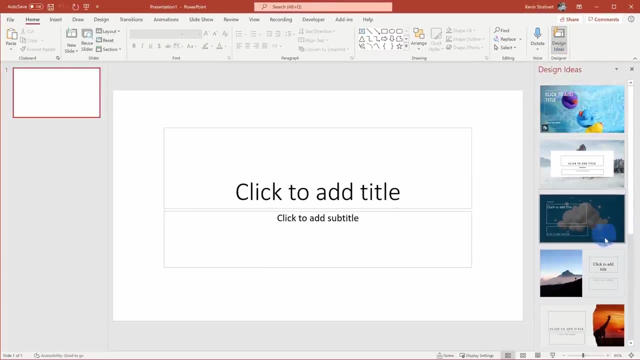 some video backgrounds. I'll show you two different ways that you can insert video backgrounds, and the first way is pretty simple. Right up here on the home tab, all the way over on the right hand side, you'll see an option for design ideas. Let's click on that If you've never used design ideas. 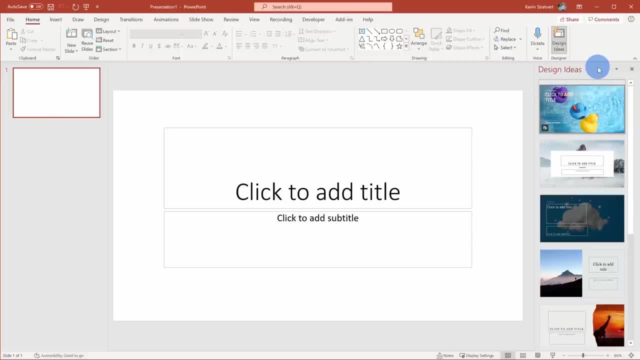 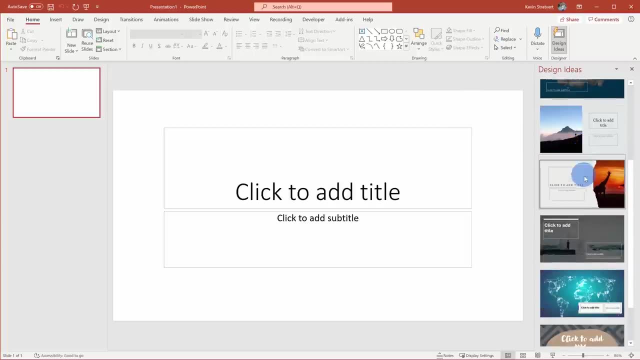 this is PowerPoint AI recommending different designs to you that you can incorporate into your presentation. It makes it really easy to create slides that look good. Here you can see just a few examples of what it's recommending or proposing to me. At the very top you'll see that.